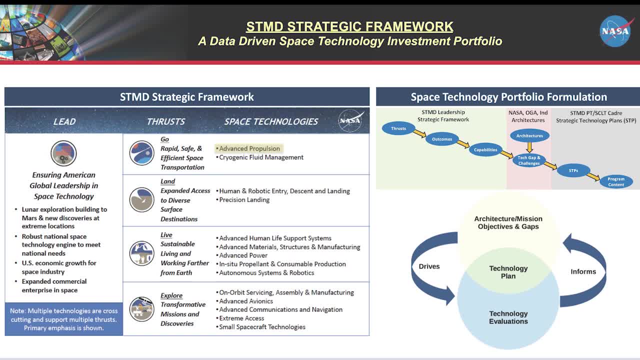 Within each of these thrust areas, there is a set of strategic technology plans corresponding to the technology discipline areas of relevance. The Advanced Propulsion Strategic Technology Plan, for example, is primarily aligned with the GOAL thrust as an enabler for rapid, safe and efficient space transportation. 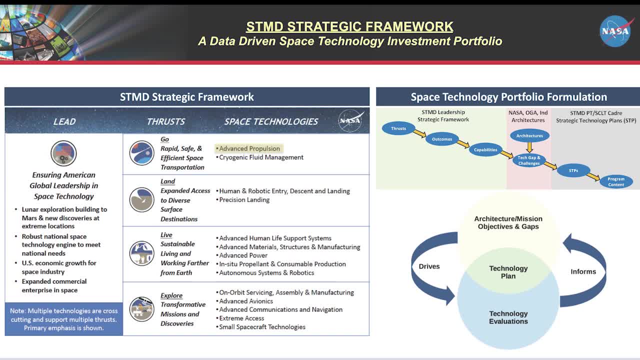 For each thrust, NASA leadership has established a hierarchy of outcomes and capabilities that align with the strategic priorities of the agency's stakeholders. These outcomes and capabilities are subsequently linked to the critical technology challenges and gaps corresponding with the desired space architecture objectives. The purpose of the disciplinary strategic technology plans is to guide the formulation of program content that will result in the closure of these key technology gaps. 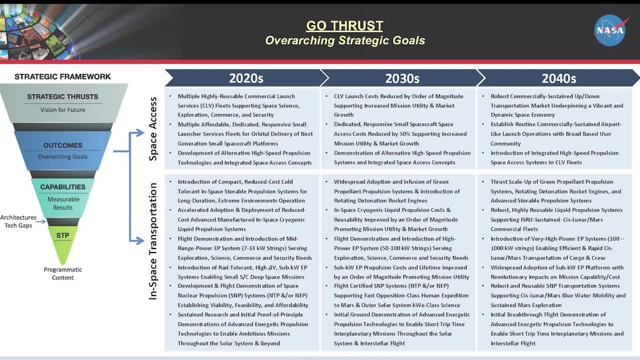 The strategic framework fundamentally consists of a long-term vision for the GOAL thrust. as shown on this slide, It is a decadal-like projection for future outcomes and capabilities. A multi-decade vision statement incorporates more information than we can cover in this brief introduction. 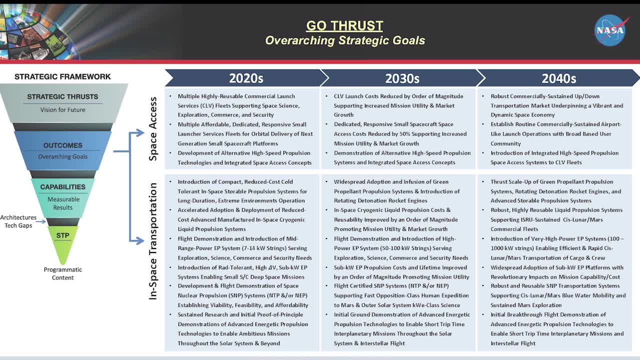 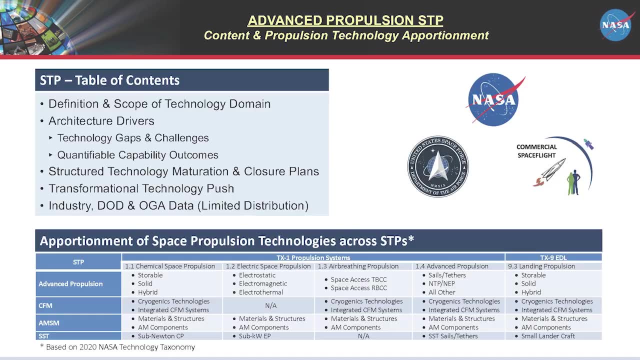 I would urge you to review it in detail at your leisure, on your own. The key point to note is that our strategic technology plans are the essential mechanism for relating these outcomes and capabilities to architecture, to ideas and to development. With this, we see critical technology gaps with direct impact on programmatic content. 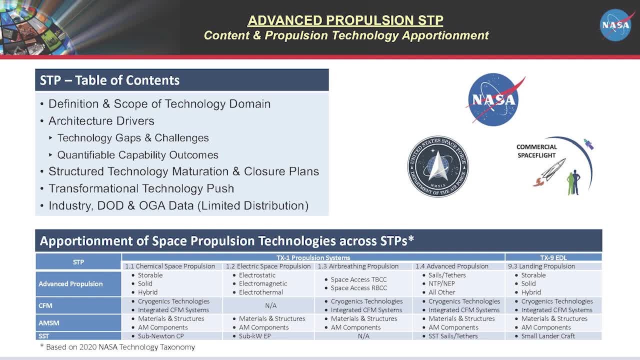 Now the content of the Advanced Propulsion Strategic Technology Plan is shown in the top left of this slide. It includes The definition and scope of technology domain, an indication of the architecture drivers from which we derive, the technology gaps and challenges, and our quantifiable capability outcomes that we need to achieve. 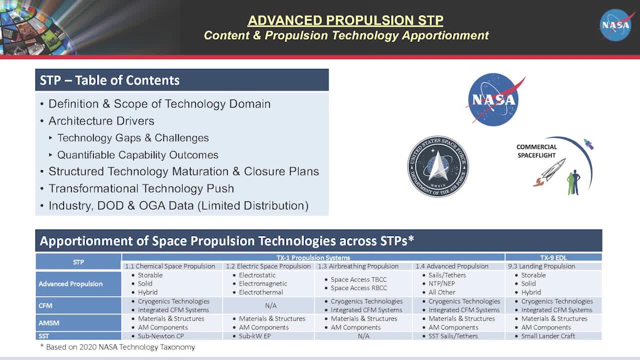 Based on these three pro Dragha things- N paralabilis and guide, designDR and ценalides, we try to integrate a global improvement model that would identify and customize the technologygent engine, These UI developments where N paralктics exist. 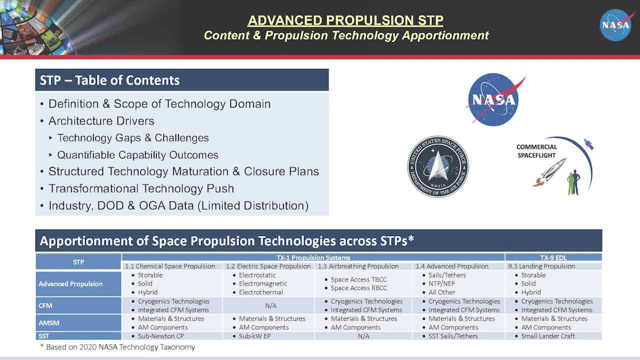 On the right you can see anisés: technology gaps and challenges and outcomes. We have the formulated structured technology moderation plans, which are intended to serve as a guide for closing the gaps. In addition, we also include some suggested research and technology investments in transformational 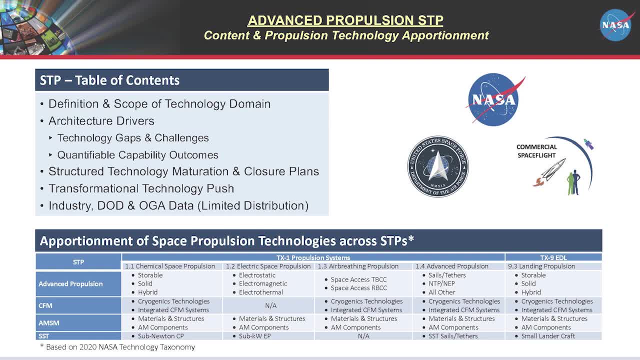 technologies. Now, our transformational push technology strategy is not meant to directly address near-term architectures, but it's intended to provide some sustained investment funding so that to pursue transformational technologies that could provide a radical- you know, transformative- change in how we conduct space transportation in the future. In addition, the strategic technology 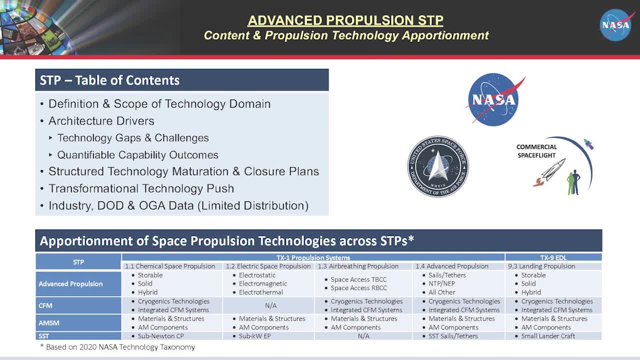 plan will include some content on industry and DOD and OGA data to provide data on the current activities across the nation in the industry, in the private sector and within the government. The idea is here to to more, better understand and coordinate our activities in relation to the activities in other organizations so that we more we can more effectively manage in. 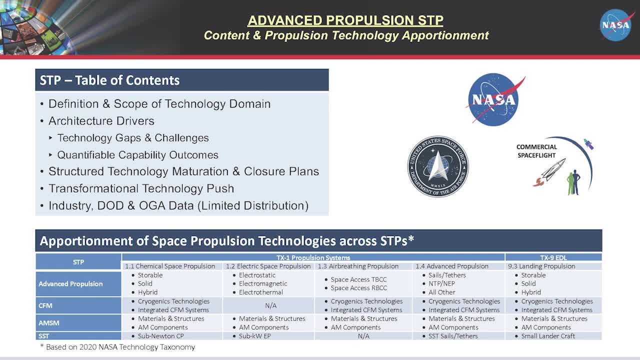 our resources and outlays. Another point to take and remember is that when looking at these plans, that the space propulsion technology is also included in plans beyond advanced propulsion plan. For instance, there are portions of the cryogenic fluid management plan and the advanced material structures and manufacturing plan as well. 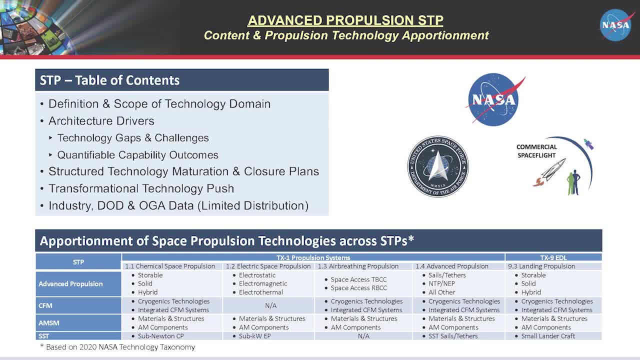 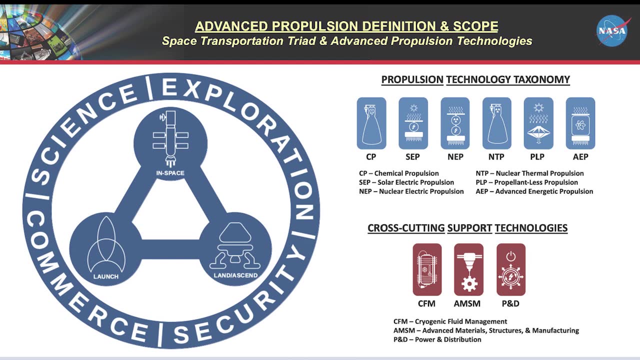 as the small spacecraft technology plan, which incorporates some aspects of propulsion which may be of relevant interest to you, so I would urge you to consult those plans. in addition to the advanced proposal plan, This next slide conveys the definition and scope of the advanced propulsion domain. 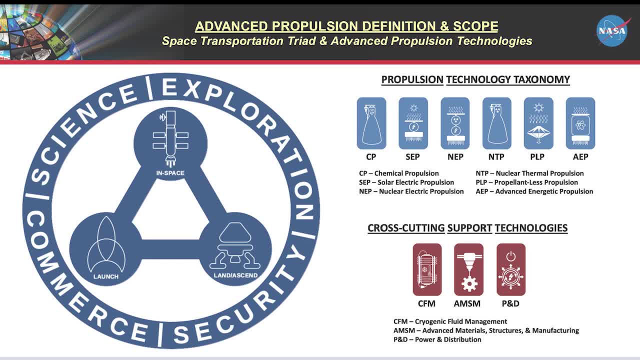 Second slide is a example of what the F läpöthey put together. The icon on the x: basically it represents first of all the space transportation triad. Propulsion technologies must support the entire spectrum of transportation systems, including launch in space and land and ascent on planetary bodies. so essentially the transportation triad. 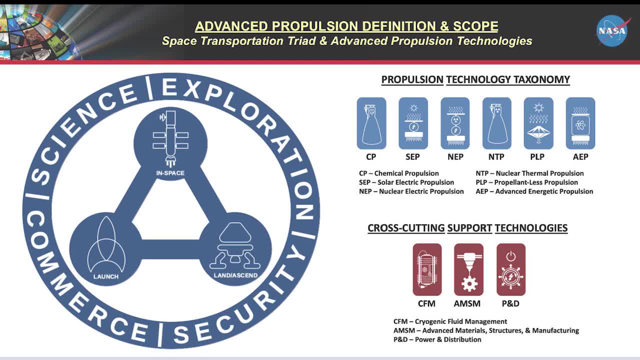 represents all of the transportation, space transportation systems Which propulsion technology must address. It's an all MOOTIS program. it's really easy for ours to do this and that, If you look at the icon, you'll also see that there's a circle representing the different 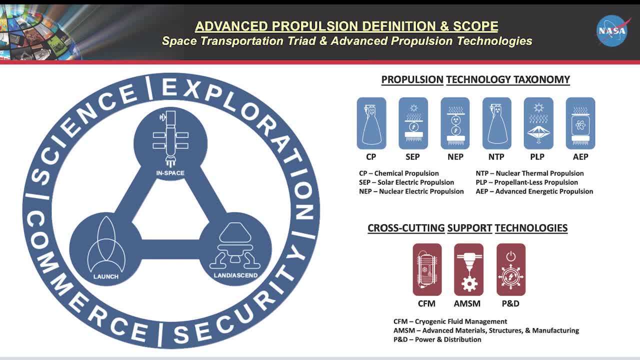 architectures which the transportation systems must support. So traditionally, NASA has focused on science and exploration. Now, currently, we are moving toward an agenda where commerce is becoming an available part of our plans in the future, And I would also ask you to recognize that space security is something that's growing. 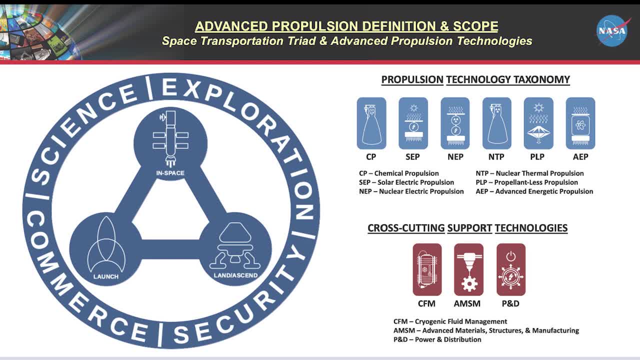 and of growing importance, and there are many dual use applications where propulsion technology that are useful for science and exploration will have implications for space security architectures as well. So all of these architectures need to be considered as we're addressing advanced propulsion technologies, And the icons on the right hand side are just meant to represent the propulsion technology. 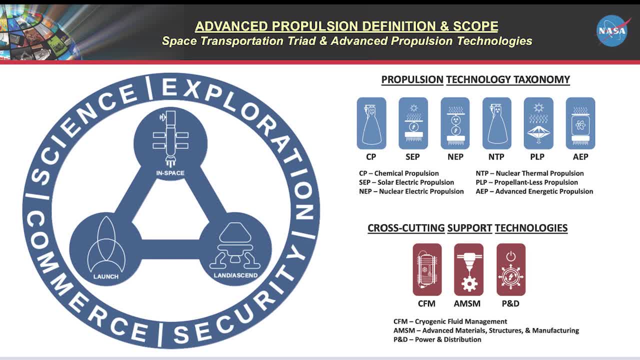 taxonomy that's being utilized in this technology plan. I think you'll recognize most of these from your past experience. They're very conventional. We have chemical propulsion, solar electric propulsion, nuclear electric propulsion, nuclear thermal propulsion, propellant propulsion and we have a category which we call advanced. 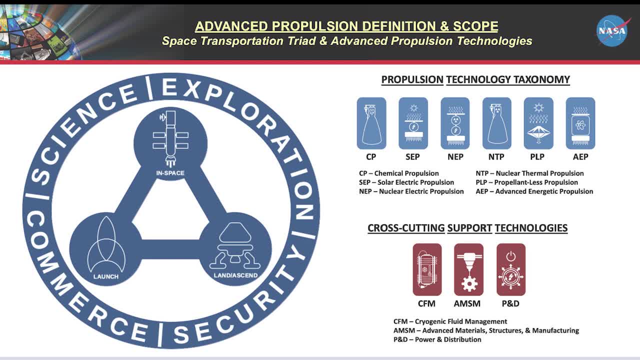 energetic propulsion, which is essentially intended to capture advanced nuclear systems beyond NEP and NTP. In addition, propulsion systems rely on a number of supporting technologies, So there are cross-cutting support technologies that are really important in terms of propulsion technology, and they're indicated in the bottom right icon collection. 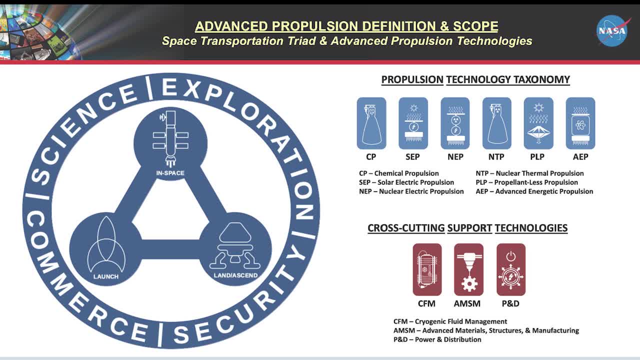 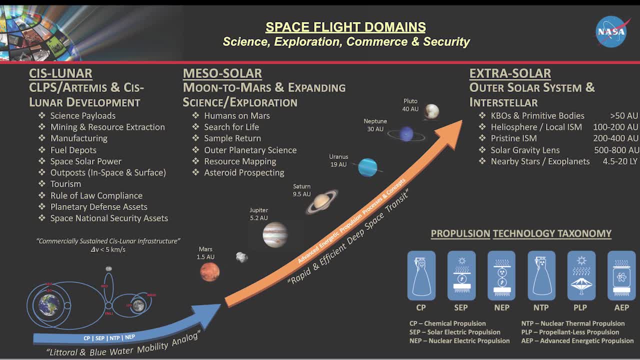 And those are projects that include management, advanced material structures and manufacturing, and power and distribution. The next slide represents the spaceflight domains that we are considering in terms of science, exploration, commerce and security. Now, in the near term, the focus is primarily on cislunar. 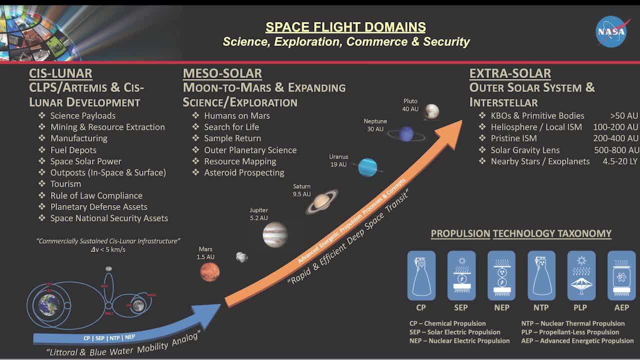 There are a number of applications in the spaceflight development for Eclipse Artemis programs in particular, And if you look at this slide you'll see a number of application, mission applications and commercial applications and security applications that people have in mind in the 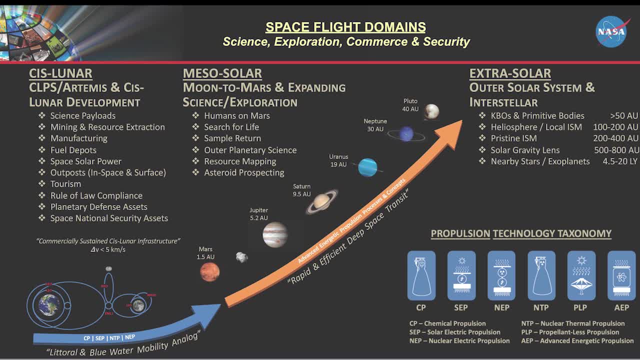 cislunar environment And largely these can be supported with a modest depth of view requirements. So chemical propulsion and solar electric propulsion can largely support the cislunar development activities. As we move out toward Mars, however, in the Meso-Solar region we're going to see a lot. 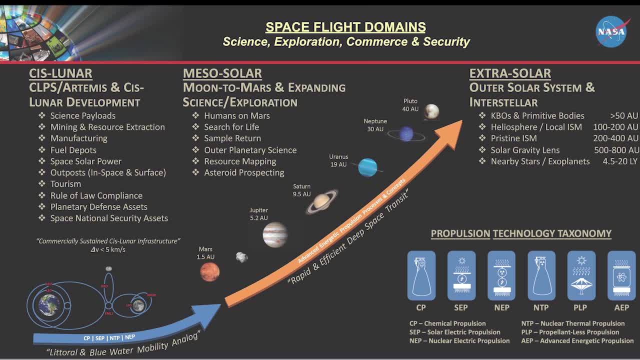 of things We're going to see: energy, what we're talking about: humans on Mars, search for life, sample return from planetary bodies, more in-depth outer planetary science and resource mapping. We find ourselves being a real need to move toward nuclear systems. 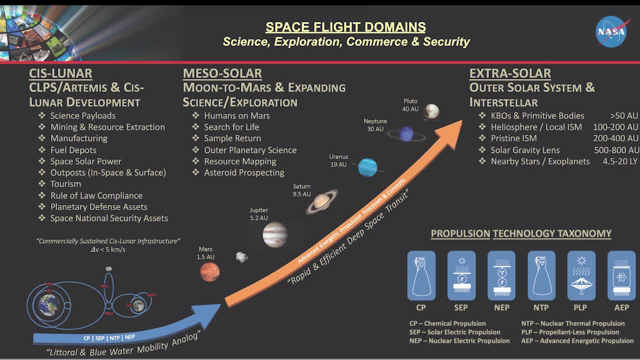 So the strategic technology plan for advanced propulsion. a large part of it is addressed at future nuclear systems such as nuclear propulsion, nuclear electric propulsion, which will begin to provide us the littoral and blue water mobility type analog systems. The other key thing that we'll be doing is to apply the 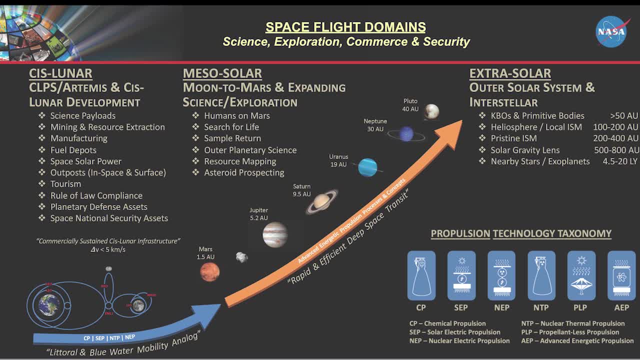 synopsis of the system, which is the intergenerational transportation capability. We will need to support that agenda. As you move out further toward extrasolar, the really far outer solar system, and stellar, the distances become so large and the Delta V requirements become so large that really, 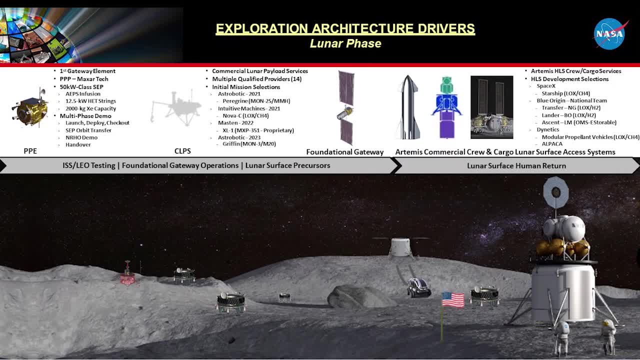 you're really forced to consider advanced energetic propulsion processes and concepts beyond NEP and NTP. So that forms a part of our transformational push technology strategy. So the next slide. few charts talk about architecture drivers, and the first one i'm showing here is for the lunar phase. 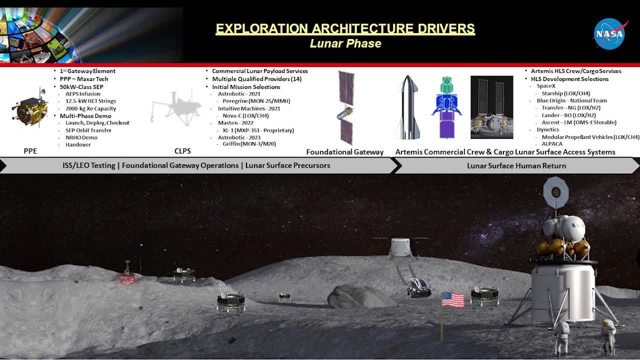 uh, the different uh drivers that we're supporting. one is the propulsion power element, which is the first gateway element. uh, we're working diligently on solar electric propulsion for that uh, for that element. yeah, this is followed by the commercial and payload services, uh vehicle systems, uh, there. 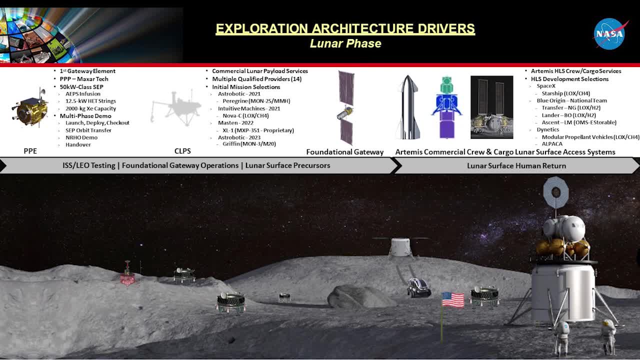 is a number of systems that have been uh that are being developed and then missions that have been selected uh for the lunar payload delivery we uh there are a number of technologies that are needed to enable those uh clips, uh uh vehicles, and we're- stmd is working uh on technologies on those uh. 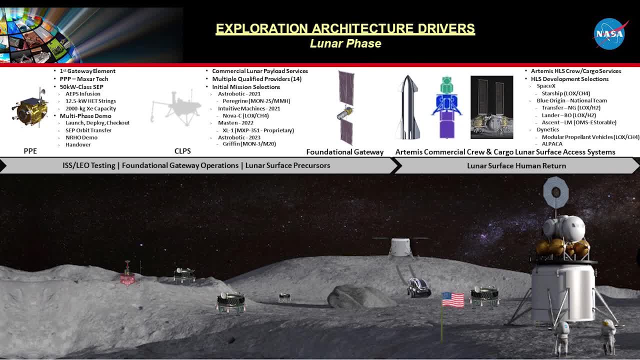 developing those technologies, support those clips systems and for human, for the art of this program there, the, the transportation systems are essentially under a crew cargo services, uh uh, similar to clips uh, and this is all under the hls uh program. uh, if you, you'll probably recognize that. 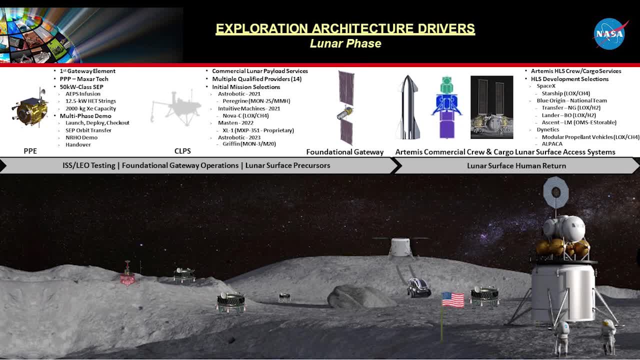 the number of arc. there have been a number of architecture development selections, uh including spacex with its starship. uh locks methane through origin national team for transfer lander and ascent using cryogenic propulsion and storable propulsion technologies, as well as dynetics, which is uh utilizing the locksmith and cryogenic. 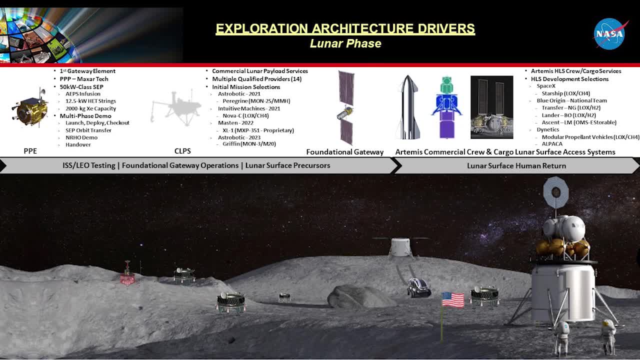 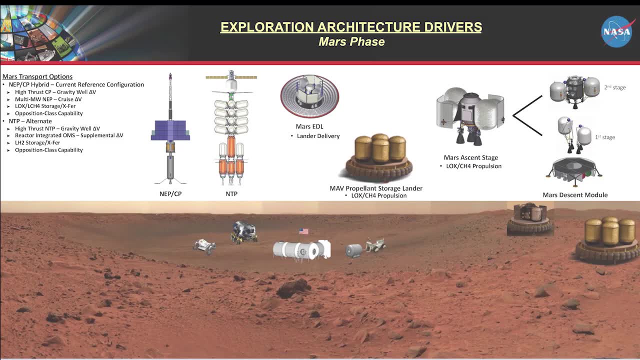 uh a variety of propulsion technologies uh, including their alpaca concept. so those are the drivers for the lunar phase uh. the next chart talks about the mars phase drivers. uh, essentially, we're for mars transport, for crude mars transport. there are two primary options under consideration. one is the nuclear propulsion, chemical propulsion hybrid, which is: 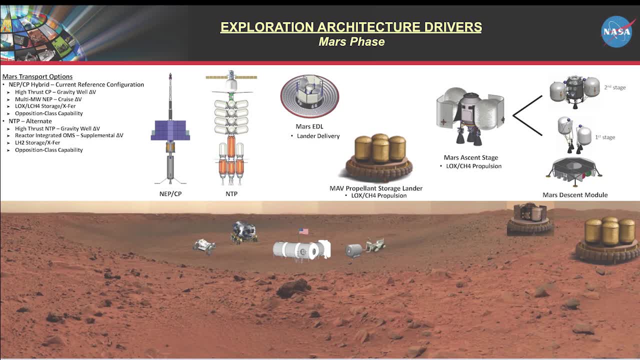 our current reference configuration is shown on this slide and the nuclear thermal propulsion is an alternate uh configuration which we are considering as an option. both of these systems are capable of doing fast opposition class uh capability. in addition to the in-space uh transport systems we have, we are looking at mars edl uh technologies for lander delivery. 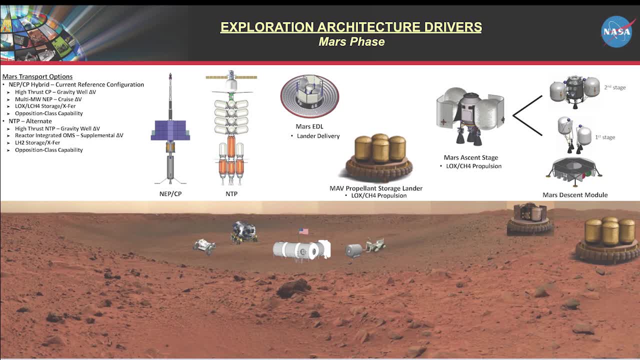 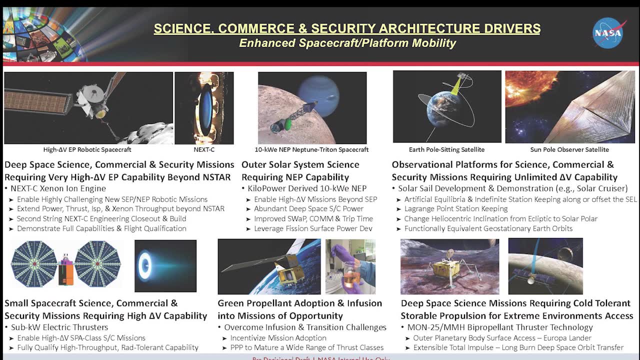 and cryogenic propulsion technologies for the various landers and assist stages which will be needed to support the human mars expedition. the next chart talks about the the uh science, commerce and security architecture drivers. uh, there are six total here and they're essentially concentrated on enhanced spacecraft and platform mobility. uh, we don't have time within this brief. 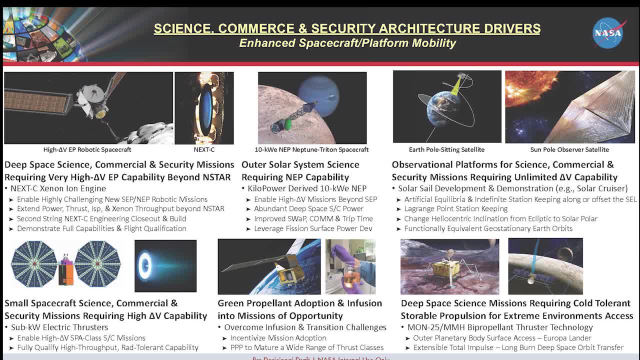 introduction to go into those in in detail, but i i would ask you to uh read those uh at your leisure and become more familiar with them, because i think these are going to be the the primary areas where we will be interested in investing in technology development to support those. 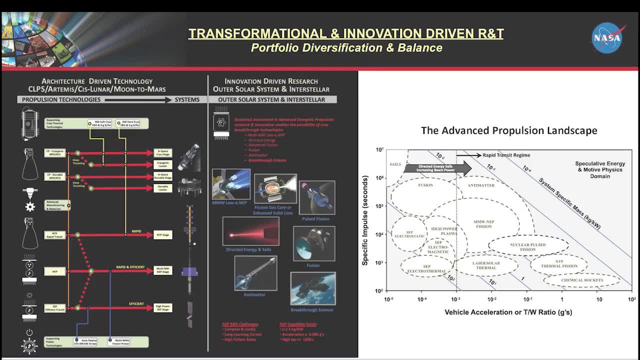 architectures. this next slide uh is to give you uh some idea of about our transformational and innovate innovation driven rnt plans. uh, most of our efforts are going into architecture: different driven technology for clips, artemis, sicilian, or moon to mars, as shown on the far. 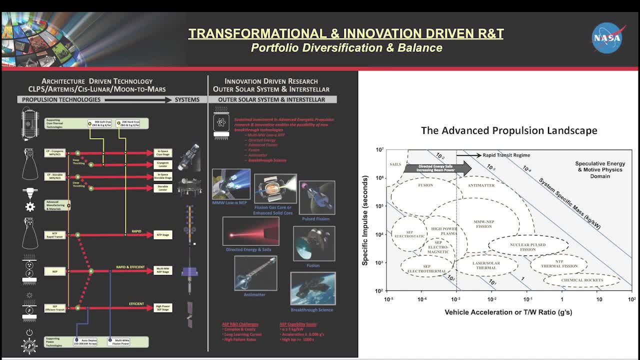 left of this slide. but we also, as i mentioned earlier, want to have some sustained investment in innovation driven research to support outer solar system and future interstellar missions. middle of the slide and advanced propulsion. uh, to give you an idea of the type of systems we're talking about, you can look at the advanced propulsion landscape figure. 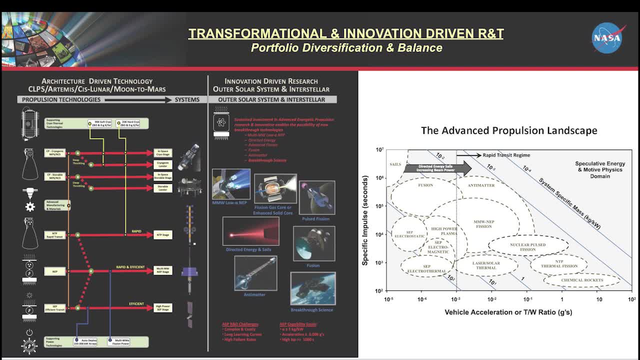 on the far right and basically it shows you that we're seeking a pretty for rapid transit. we're trying to achieve vehicle accelerations or thrust to waste ratios greater than 10 to minus 3g and if you examine that, that, that chart, you'll see it drives you to advanced nuclear systems largely. 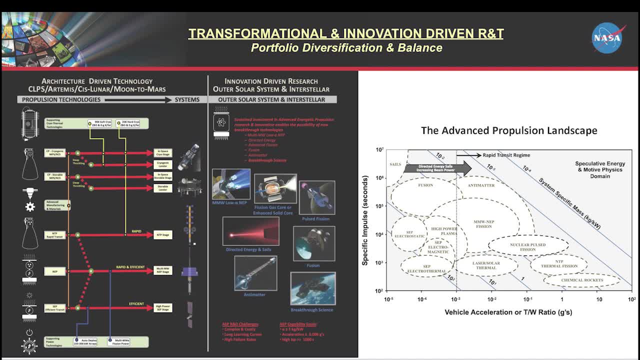 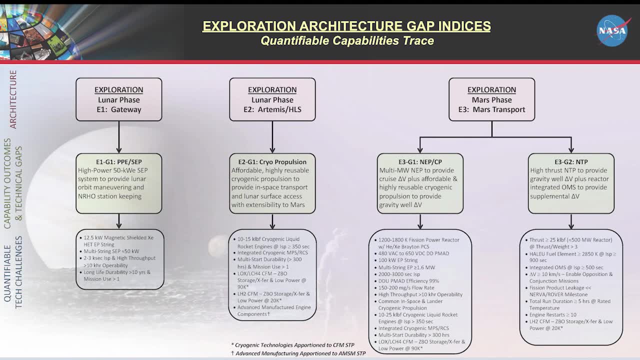 that are that are well beyond what can be accomplished with uh, nep or ntp. so these are truly advanced energetic propulsion technologies. the next few slides are going to talk about the, the architecture gap indices that we've developed, uh that include quantifiable capabilities, traces to the perform key performance metrics that we need to achieve. so the first one here, slide i'm 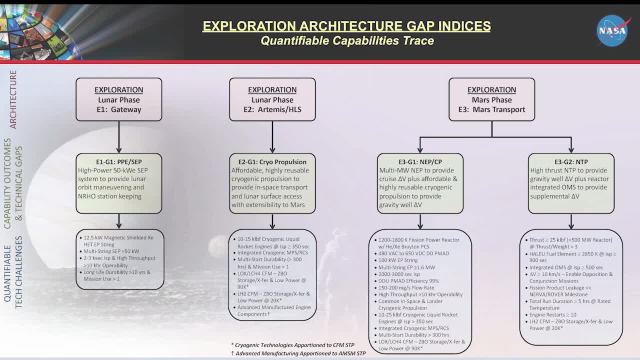 showing you is on the expiration architecture and it identifies the expiration uh technology gaps for the both the lunar phase and the mars phase, and they've been. the indices are indicated for reference purposes and if you follow the trace for each of those uh gap indices, you will come to a a short description of the capability outcome. 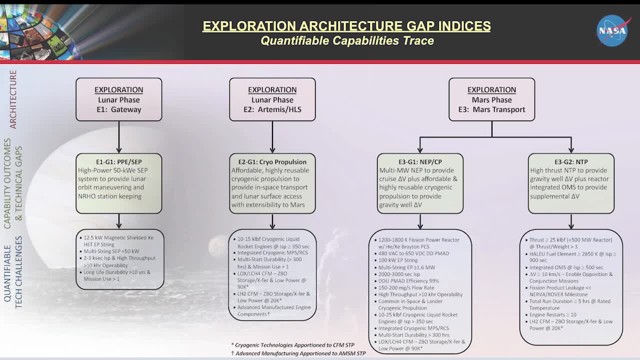 and technology gaps that we're addressing and if you follow the trace down to the bottom, you will come to the key performance metrics that we need to achieve in order to close the gap and enable the architecture of interest. uh, you will see that the mars transport capabilities trace does have a split in it, and that's because 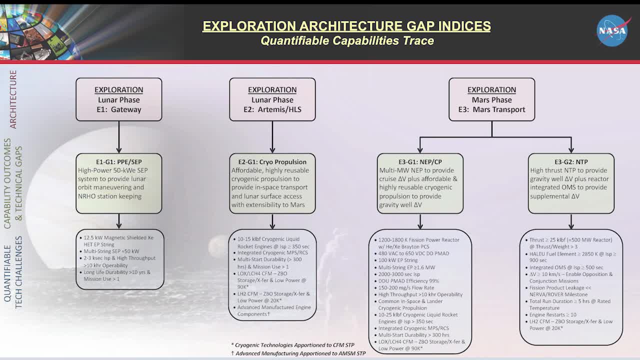 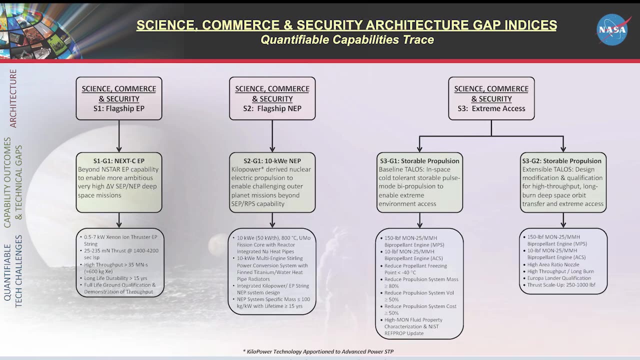 we have not made a decision on whether we will pursue the nep compulsion architecture or the nuclear thermal propulsion architecture. so for the time being, both of those architectures will be pursued and we'll be pursuing investments to close the technology gaps for both of those architectures. the next slide discusses uh. 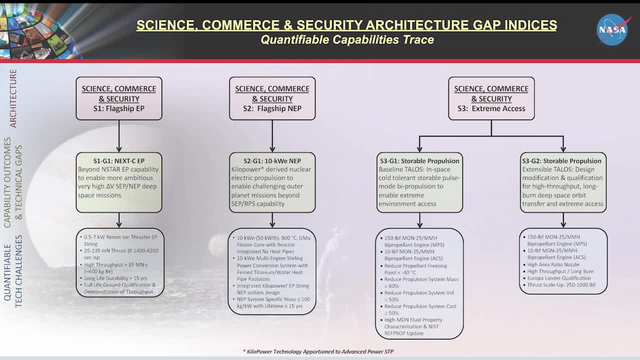 science, commerce and security architecture gaps. so we have the indices identified here, uh three of them for three of the architecture gaps: uh one for flagship uh electric propulsion, another for flagship nuclear electric propulsion and another for extreme uh access uh concentrating on code tolerant propulsion. so in a similar reason, there's a similar capabilities trace for each of those. 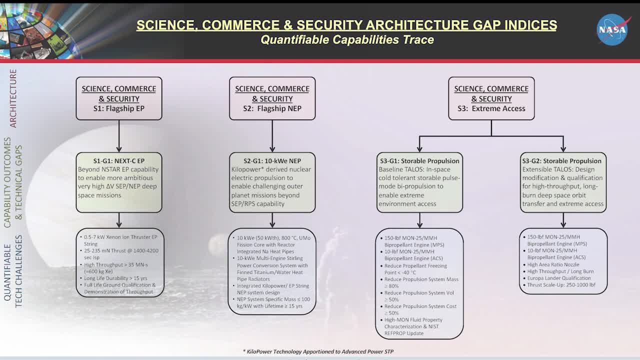 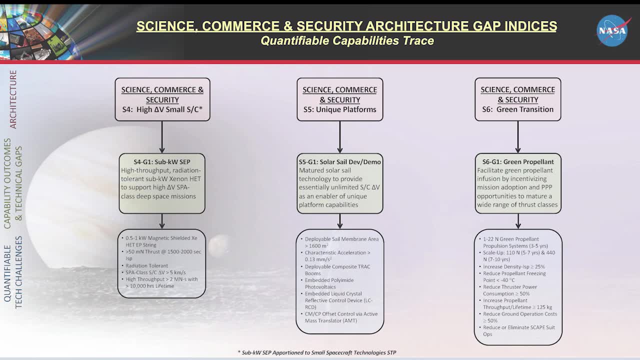 gaps. i'll leave you with you to investigate on your own. the next slide is is the remainder of the science, commerce and security gap indices. the first one is for high delta v small spacecraft propulsion. so this is sub-kilowatt solar electric propulsion that would enable uh, esp class, uh type of small spacecraft missions. 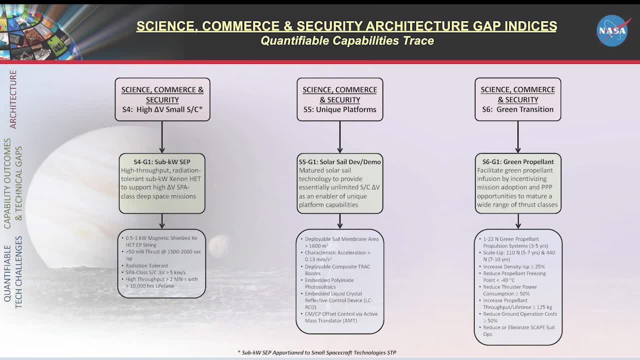 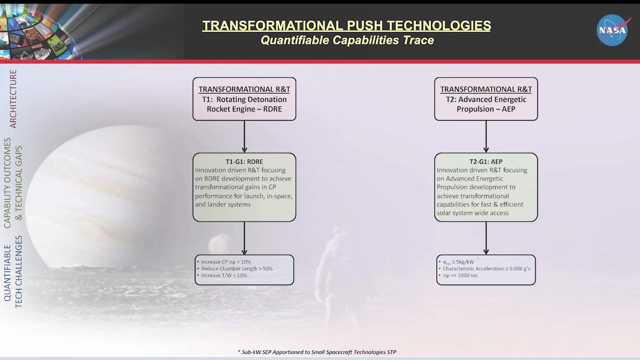 science missions. uh. there are unique platforms, uh. uh gap indices for solar cell development and demonstration and the final uh gap indices for green propellant trans transition, where we're trying to encourage, facilitate and encourage the adoption of green propellant uh technology. uh for future science missions and the. the last uh quantifiable capability traces is for: 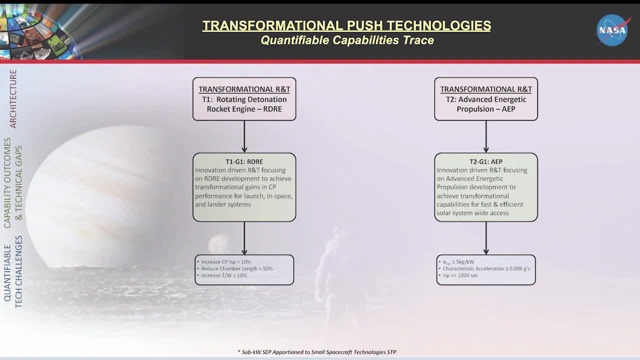 transformational push technologies. i have two identified here. uh, the first, transformational rmt. a focused investment is is on rotating detonation detonation rocket engines. These are. this is a technology that offers a lot of promise with a lot of risk, but it could truly transform. 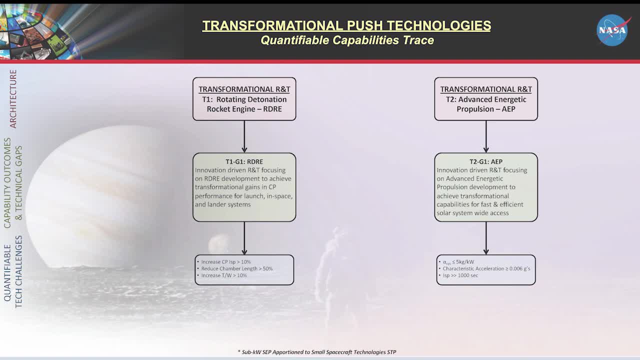 the way we do future in space transportation, So we would like to maintain some sustained research and technology investment in that area. The other transformational research and technology area that we would like to invest in is advanced energetic propulsion, As I mentioned previously, as you move further and further out from the Earth. 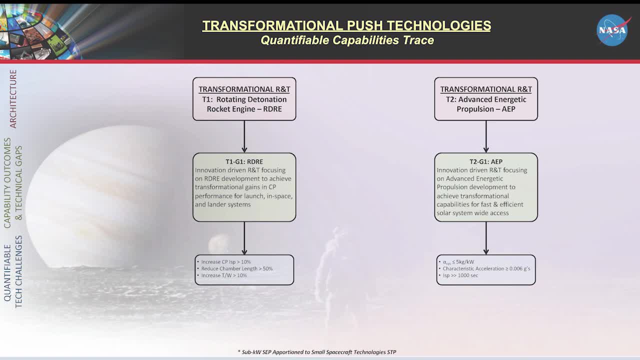 and further and further into space. the Delta V requirements and the distances involved really push us to some type of propulsion technology you need that is beyond conventional nuclear thermo propulsion or nuclear electric propulsion capability. So this is another area of a transformational investment. we would hope to sustain some investment. 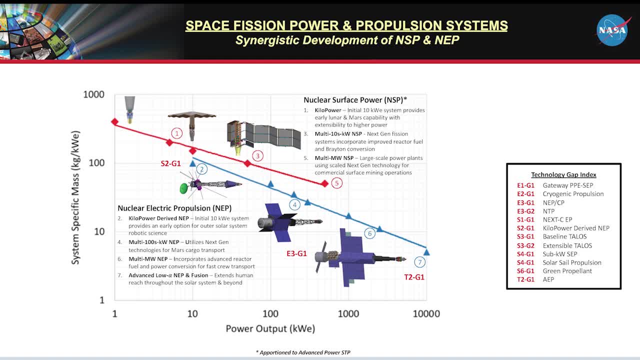 The next slide just quickly shows you the overlays, the technology, the evolution that we perceive for nuclear surface power in comparison to nuclear electric propulsion, And the point here is to show you that there's a very synergistic development strategy that can be put in place. 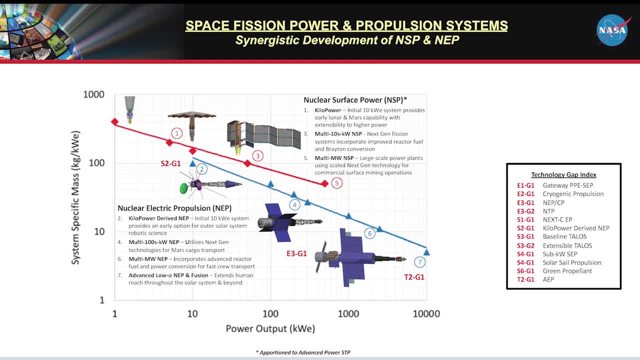 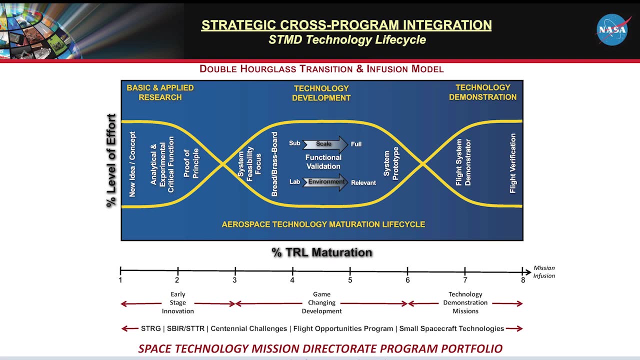 when we're developing nuclear surface power and nuclear electric propulsion. These are very synergistic power systems, So it's of much we can leverage when developing one to benefit the other. and the next slide that I'm showing you is beginning to talk about our strategic cross-program integration strategy. 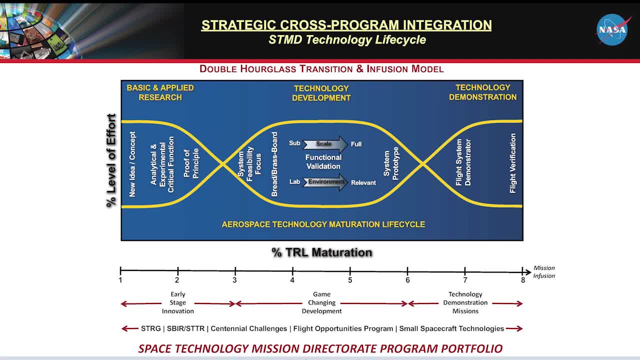 The first one here represents the space technology mission directorate technology life cycle. The thing to keep in mind for the space technology mission directorate is we're a is a collection of multiple programs and each of those programs essentially focus on a certain tend to focus on a certain TRL range. So we have our early stage innovation programs, which 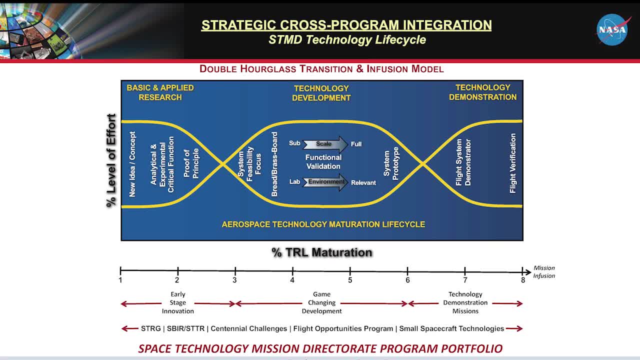 tend to focus on TRL up to three, A game changing development program, which is intended to focus on technologies that are in the three TRL three to six range, and and our technology demonstration mission program is primarily directed at technologies that really need to be flat demonstrated before they can be successfully. 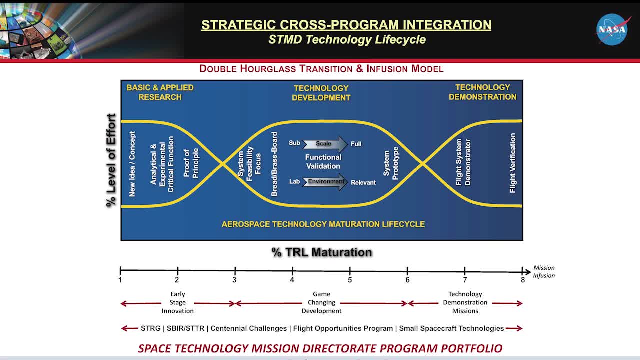 uh infused and adopted for for actual missions and some of the specific programs that are how they relate to those TRL levels are shown on the bottom and and, and some of those go across the entire spectrum, such as the SBIR, STTR uh program, which is the primary interest of this. 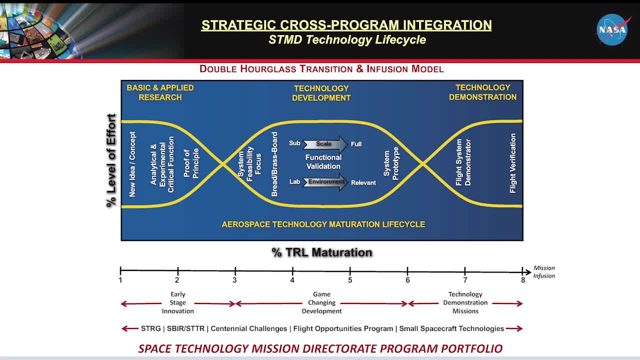 innovation and opportunity conference. So, anyway, the key point here is that one program does not care at all. we have to be very smart about how we develop our technologies and hand the program, hand these, those technologies off between programs as they technologies mature. And I want to talk about integrated program elements for a moment, because 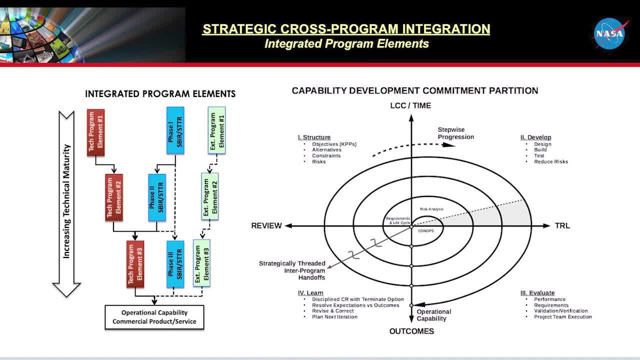 I think this is very important for for you to understand as a potential offerer of technology to the space technology mission directorate. As I mentioned, none of our programs, uh truly uh, carry a technology all the way from initial concept, the early stage uh investigation, through the mid-TRL maturation range, all the way to demo. It's a handoff from program to program as 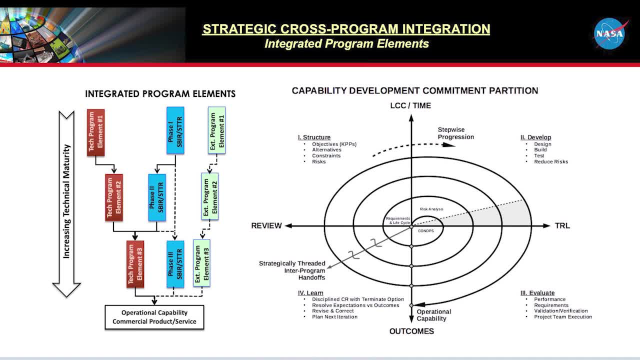 the as the technology matures, So we have to think very smart about how to utilize the STMD programs uh and and not only in sequential way but in a parallel way. So this chart is an intent, uh, to convey how we might be able to do how we envision we can do that. On the left, you can see that you. 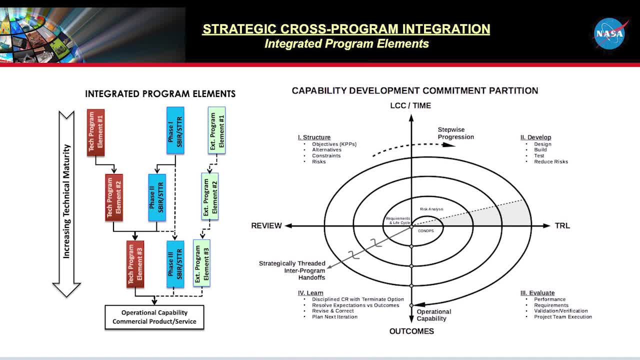 know we're trying to increase the technology. We're trying to increase the technology, We're trying to increase the technical maturity, going down, uh, until we reach an operational capability or commercial product or service of need. that we objected. And so, as you can see, as we initially 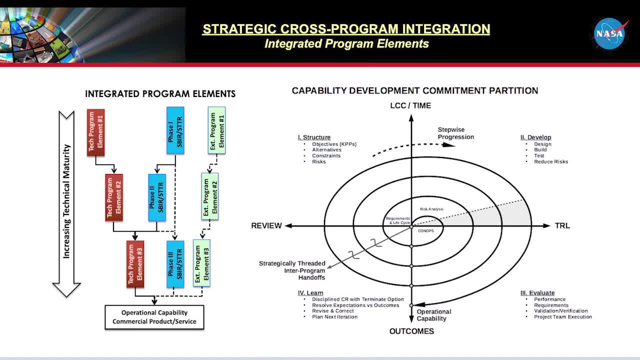 start our technology. here we may have a tech program element that is internal to the, to NASA. This may be tied to a parallel element in SBI or STTR which is providing some contribution to that technology need, And there may be external program elements that also contribute and all of these are going on in parallel aimed at a 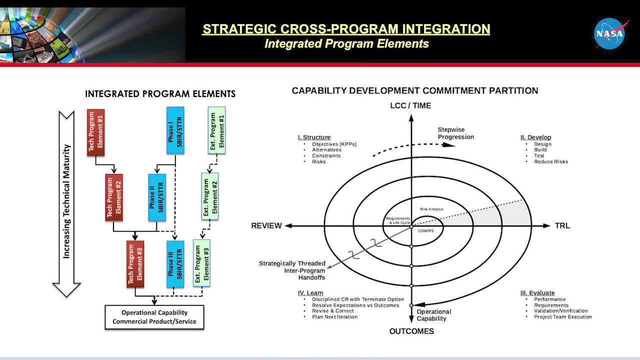 an operational end game capabilities. And so, as you can see, as those programs mature, the TRL is envisioning that they would hand off to the next level, uh, in the sequence, uh, another program element in most cases, and which would also proceed in parasail, in parallel, until you. 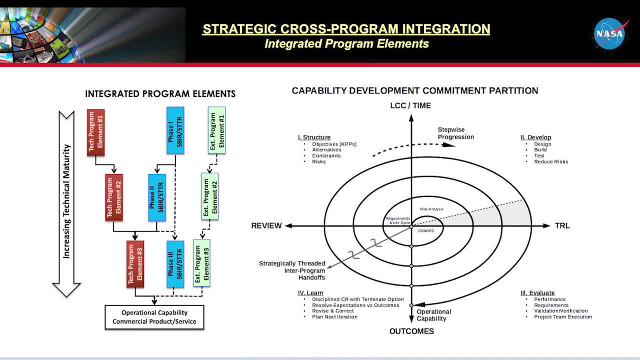 get to the point where the technology is matured enough that you've integrated all of all of the these different elements into a final operational capability, And the little diagram on the right is just, uh, essentially a capability development commitment partition that's meant to convey this.